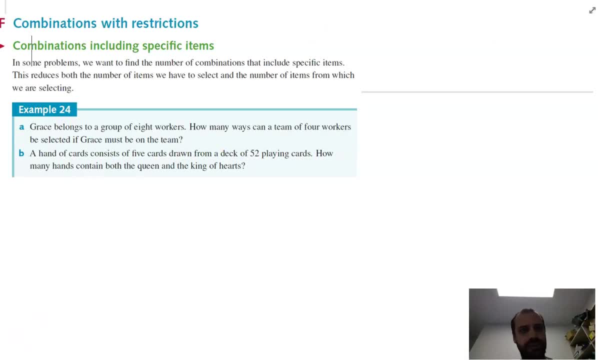 restrictions before you start. So first question here, let's just jump straight into them. Grace belongs to a group of eight workers. How many ways can a team of four workers be selected if Grace must be on the team? So that means that there's eight people in a line and we need to. 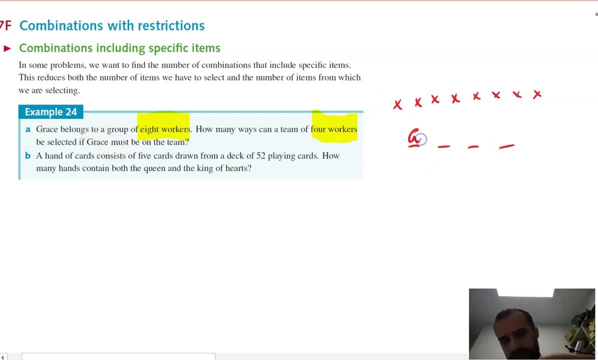 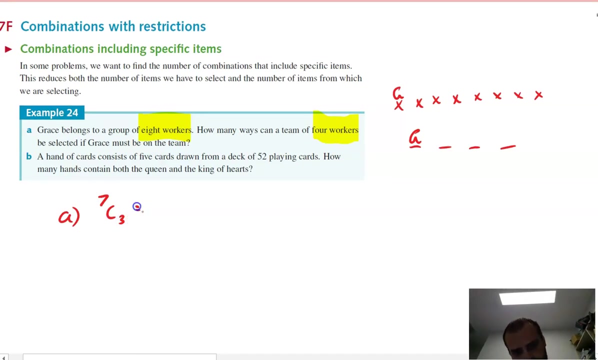 choose four. but Grace has to be on the team, So we're only choosing three people from this group, essentially because Grace was one of the people in that group. So we're choosing three people from a potential selection Seven. So the answer to part A here is going to be: seven: choose three. So that's going to be. 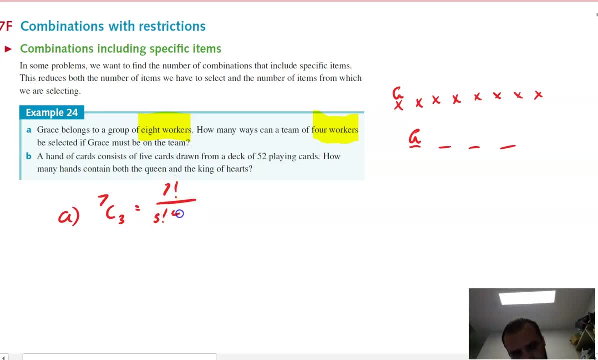 seven factorial over three factorial, four factorial. Okay, reading the next question here not going to be much different. here, I think A hand of cards consists of five cards drawn from a deck of 52. How many hands contain both the queen and the king of hearts? So we need to know. 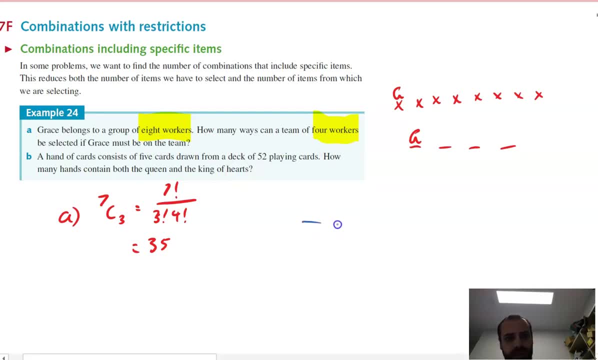 how many different hands we can have. One, two, three, four, five With a call. contain both the queen and the king of hearts, Queen of hearts, King of hearts, And then there's three extra spaces here for our thing. Now, important to note here that the queen and the king could be anywhere. 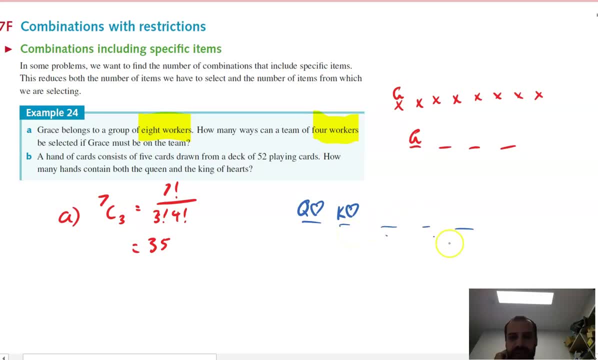 It doesn't really matter, We're just picking three extra cards. So we're picking three different cards of 40,, 50, or a potential 50. So the answer to part B here is 50 choose three. Now I'm just going to put that straight to my calculator. I'm going to get 19,600.. Really multiple. 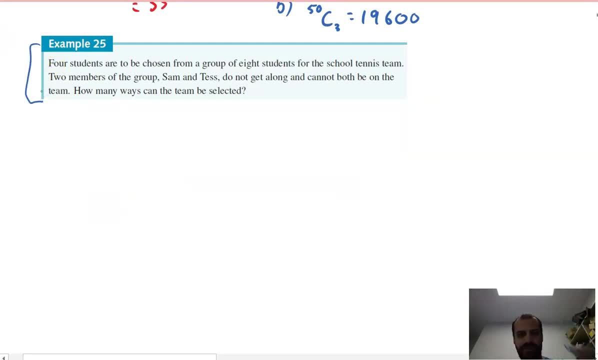 ways to get one of these questions done. but here we're going to do this question sort of in. a are to be chosen from a group of eight students for the school tennis team. two members of the same of the group, sam and test, do not get along and cannot both be on the team. how many ways can 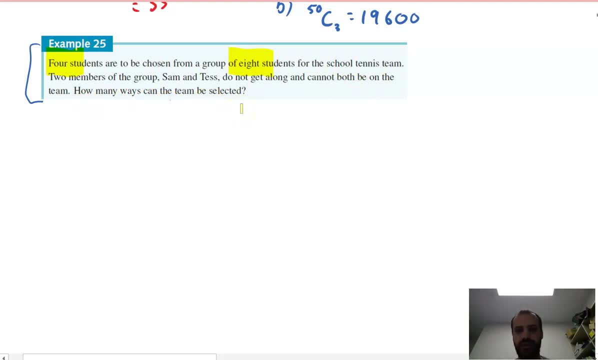 the team be selected. so i'm going to do this sort of in reverse: i'm going to find out how many, how many teams have sam and tess on them. so in other words, we've got groups of four: one, two, three, four. i'm going to put sam. 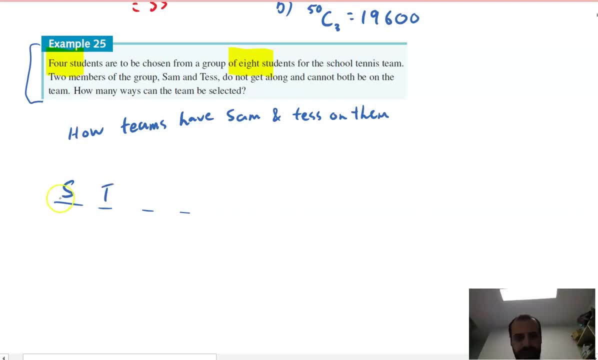 and tess on the team, but it doesn't matter where they're sitting, they're there wherever. so there's only two more people that can be on that team. um, so the way to find out how many teams sam and tess have on them is just you going to be um. so i'm going to be choosing from six, because i'm not choosing salmon tests or i'm. 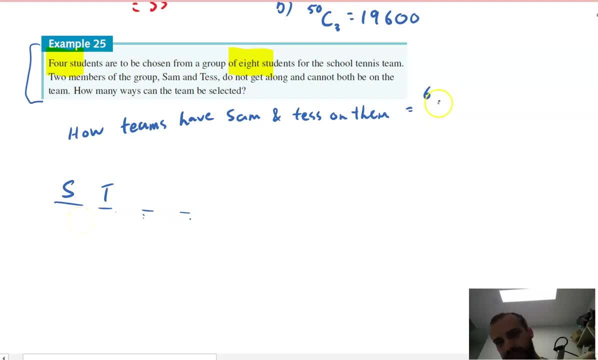 not choosing from salmon tests, because they're already on the thing: choose uh, and i'm just choosing two. six, choose two, all right, so there's 15 different teams with salmon tests on them. now, if i knew how many total teams there were, i could then subtract the salmon test teams and what i'd 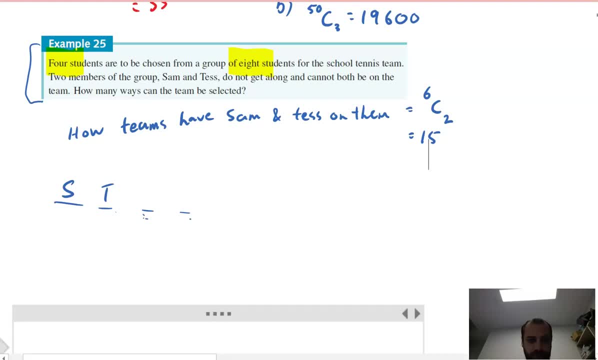 be left with is the teams without sam and tess on them. so how many total teams? well, i've got eight students and i'm choosing, uh, four students. so eight choose four, that's 70, and so, finally, how many teams don't have sam and tess on them? teams without 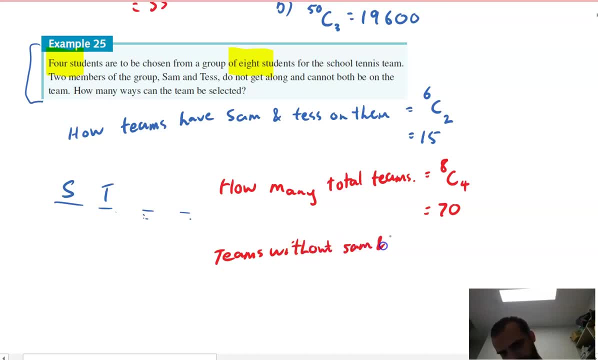 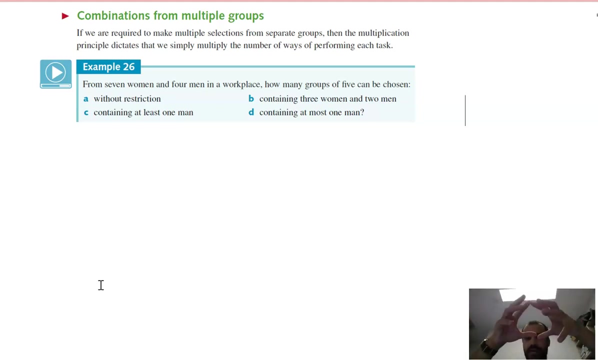 sam and tess. well, that's going to be equal to eight. choose four minus six, choose two. 70 minus 15, 55 also do, uh, combinations from multiple groups. so you've got some girls on this side, some boys on this side. you're creating one mixed netball team. let's say, all right, let's. 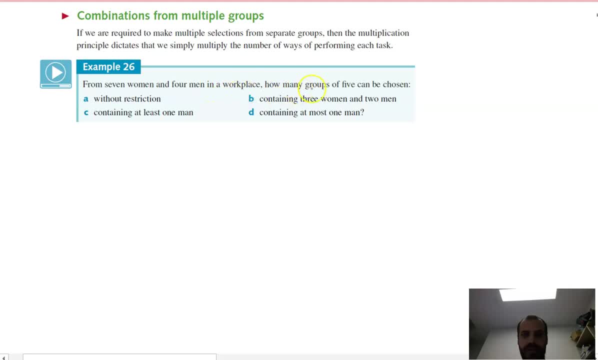 see, uh, from seven women and four men in a workplace, how many groups of five can be chosen? um? first one we're going to do is just without restriction. so it doesn't matter how many boys, you can have all boys, you can have all girls, whatever it is. so in that case we just push the. 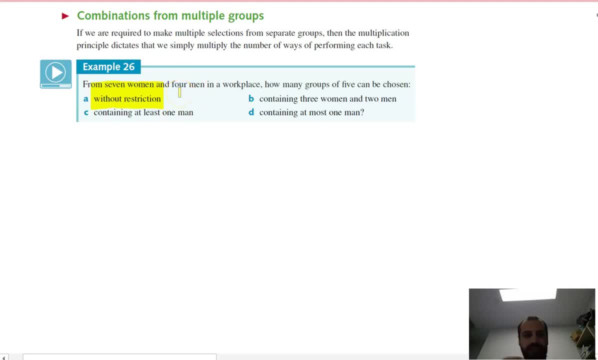 two groups together, seven women and four men, so that makes 11, and we just choose five from that 11, choose five. so this is part a. that's, uh, 462. okay. part b is where this question gets more interesting, containing three women and and two men- okay. so, uh, we need to figure out how many ways we can choose three women and how many. 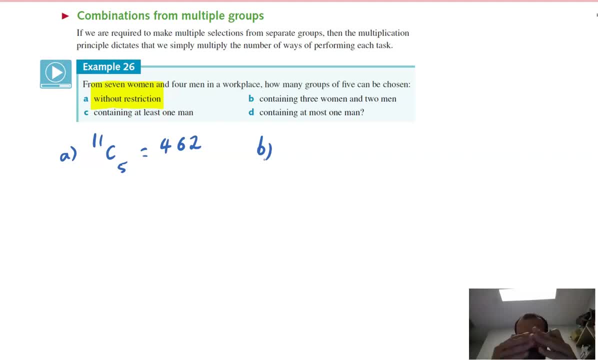 ways. we can choose two men and then we can use our multiplication principle to put those two together. uh, so it's going to be containing three women, so we're picking three women from seven, so seven choose three. so that's the women part of it, um, and we're choosing two men, so four choose two. 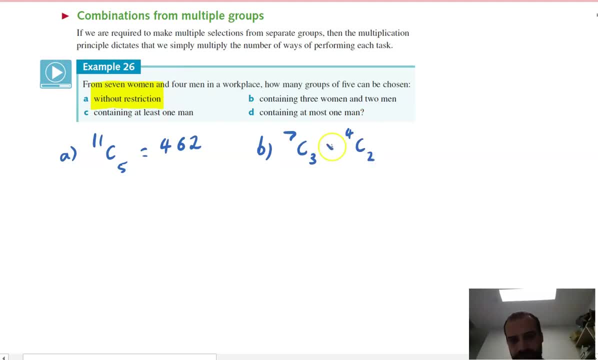 but we need to multiply them together because each of these combinations can be, uh, combined with each of those combinations, so it's a classic multiplication question. so that's at 210.. okay, um, now the next one containing at least one man. this is one of those, uh. 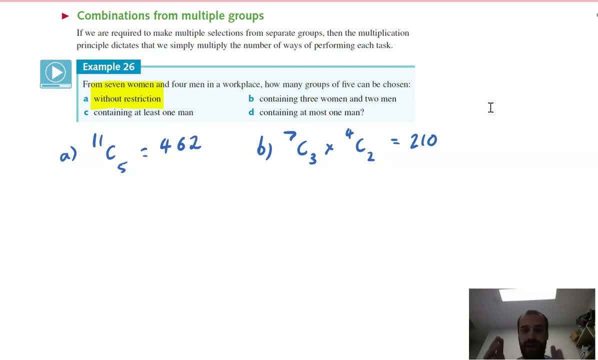 questions where you're probably better off going sort of the back, the back way, um, and just Just finding, instead of finding at least one man, finding out how many combinations there are with zero men and then subtracting that from the total combination. So we already know the total combinations. 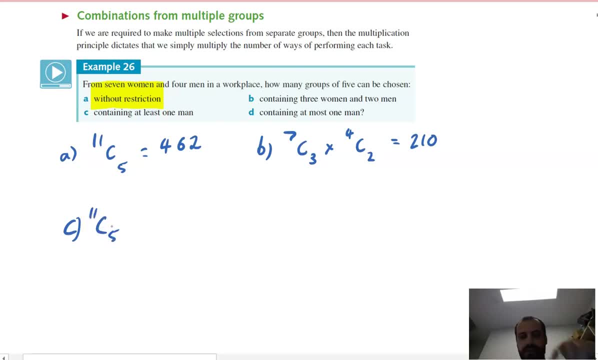 It's 11, choose five. And then we need to subtract all the combinations with no men, And so all the combinations with no men, they're all picked from the women, right? So it's seven from the seven women, choose five. 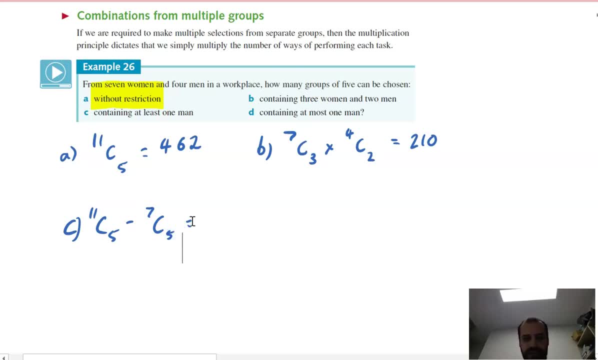 Okay, so 11 choose five minus seven choose five is 441.. I'm containing at most one man. That means we're looking for a group with either no men or just one man. So to get a group of no men is pretty straightforward. 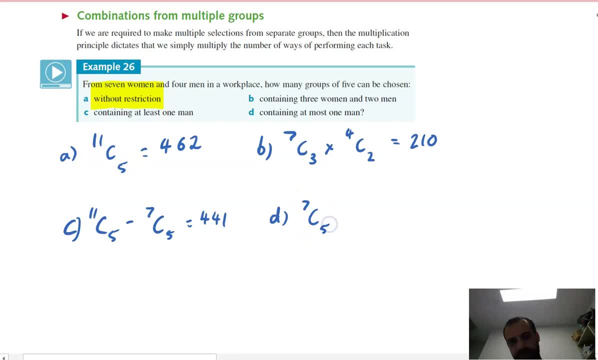 You just do seven, choose five. because you're choosing five people from the seven women And then to choose to do, just choose one man You're choosing, let's do the men first. You're choosing one man from the group of four. 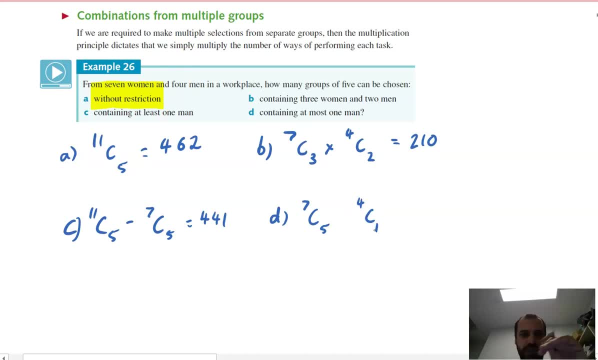 So four choose one. And then you're also choosing four women from the seven. So seven choose four, And then they are multiplied together, because each of those is can be combined with each of the other ones. But then these, these ones here, this is the addition principle. 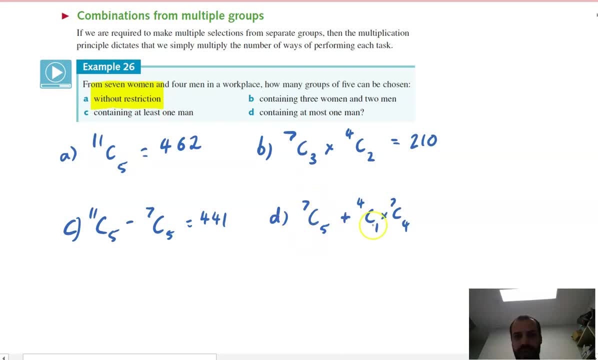 Cause these are all of the versions with zero men in them. These are all of the versions with one man in them. We can add those together. at the end We get an answer of 161.. They sometimes you might sort of have a question that combines the ideas of: 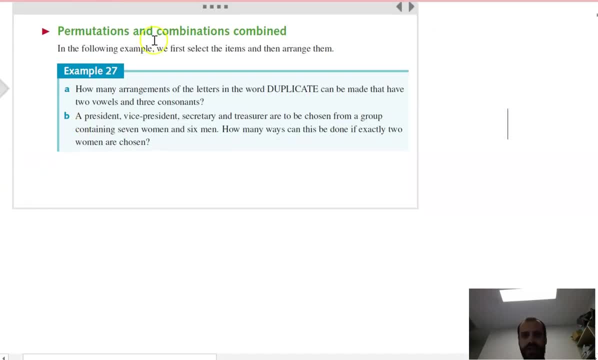 permutations and combinations with one neat little package. So let's take a look How many arrangements of the letters in the word duplicate can be made that have two vowels and three consonants. So an example of an arrangement of the letters in the word. 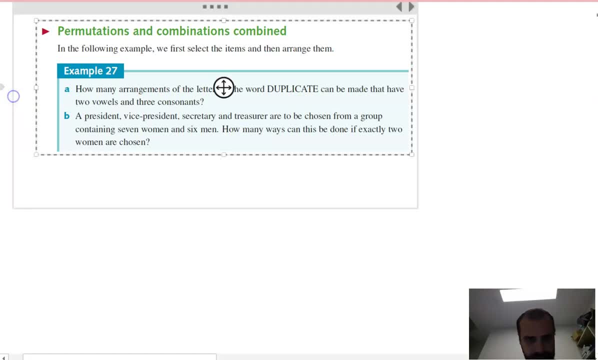 duplicate that have two vowels and three consonants is U I, that's two vowels, and D P L, D P L. another arrangement of the letters in the word that have two vowels and three consonants might be D P, L, I, U L. You can see that these are the same combination of letters. 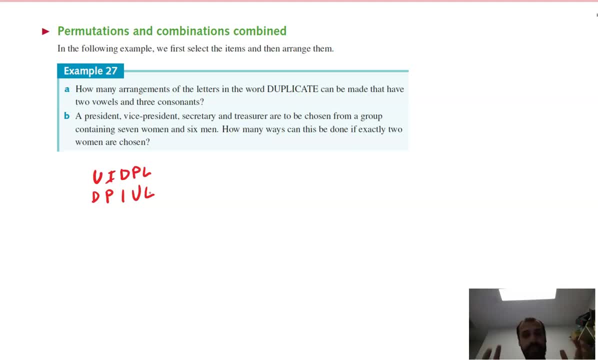 but different arrangements, Okay. So first we need to figure out how many different combinations of vowels and consonants we can get. So how many vowels are there? first There's one, two, three, four vowels, And I need to choose two vowels from that. 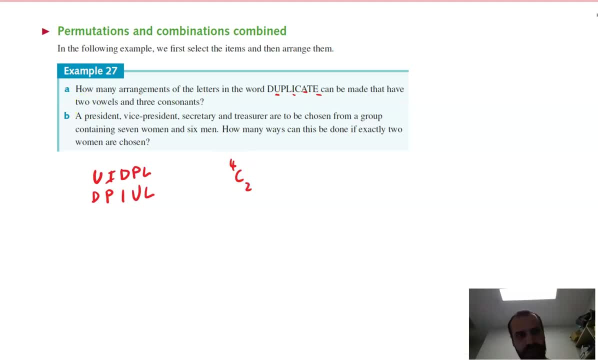 So four choose. So this bit here is the vowels. Now the consonants. let's take a look at the consonants for a second One, two, three, four, five. there's five consonants. I need to choose three of those. 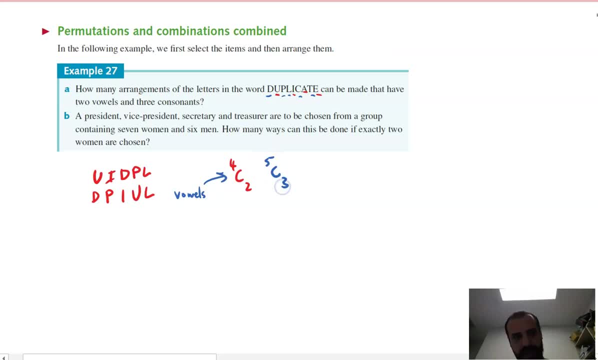 So five choose three. Now that they're the consonants, And if I multiply them together I'll know how many arrangements of, sorry, how many combinations of vowels and consonants I can get 60. But that's just telling me that, like 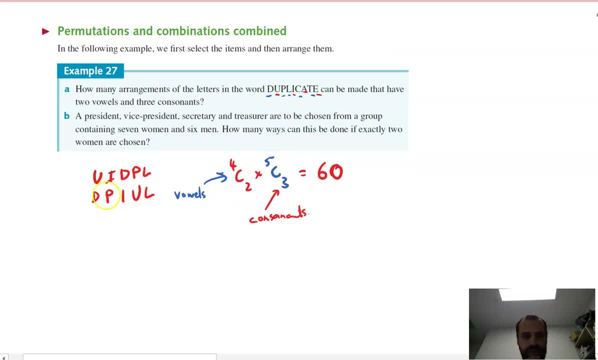 here's a group U, I, D, P, L. Now those are the same same combination, So that's not included in that. Another one might've been a I D, P, T, for instance. there's 60 different combinations, but now I need to know how many of those arrangements can I get. 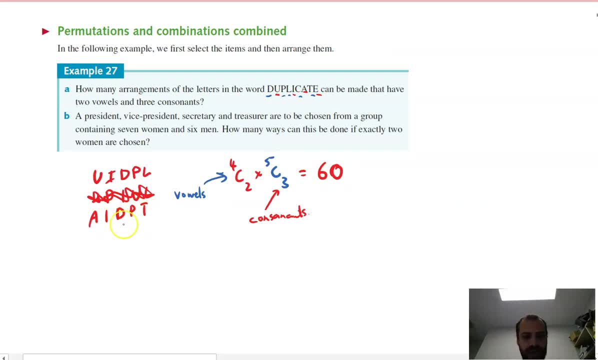 So each of those 60 can be arranged five factorial ways. So that was the combinations. So now I can take that 60, 60 times, that's 60 times five factorial. That will give me how many arrangements of those combinations there are. 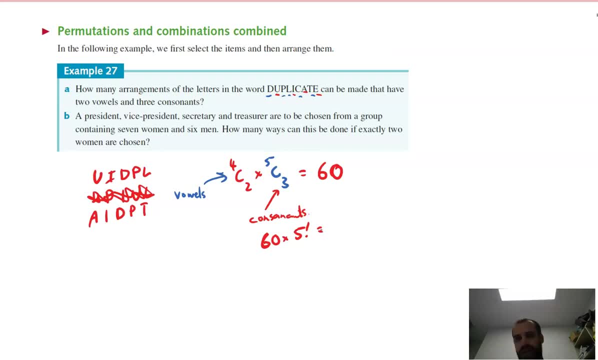 because each of the 60 can be arranged five factorial ways. So that's 7,200.. Now we can do all that just in one step. It's probably a little bit neater to say that the answer is five. choose two times five, choose three times five- factorial. 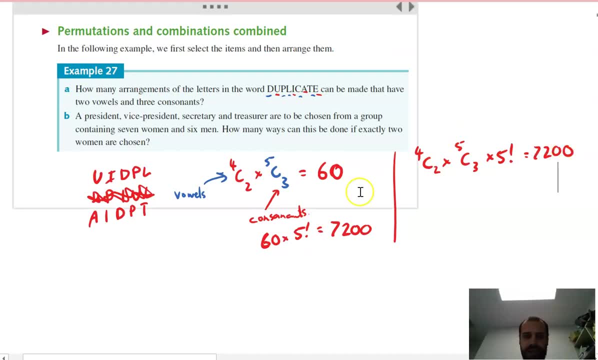 7,200.. Okay, So there's how to do a question like that. Finally, a president, vice president, secretary and treasurer are to be chosen from a group containing seven women and six men. How many ways can this be done if exactly two women are chosen? 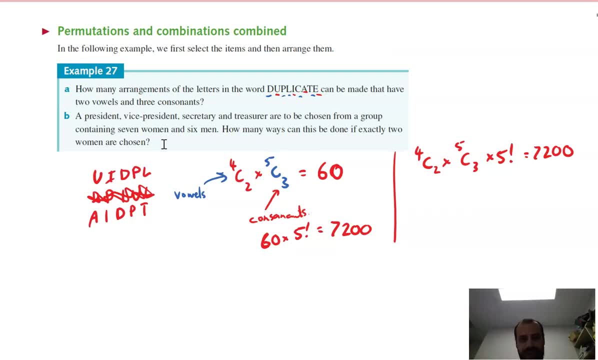 All right. So we need to find out how many ways you can choose exactly two women. So there's one, two, three, four people that we're going to choose, And we're going to choose from seven women. seven women there. 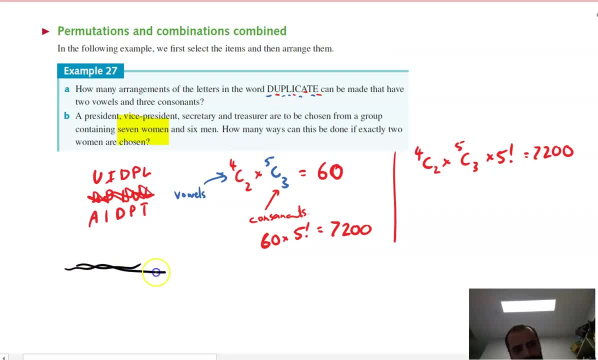 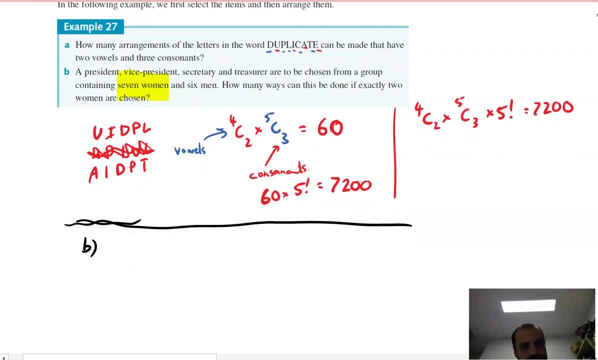 So in terms of- I'll just do a line here, So we'd know we're doing part B- So in terms of the women, first of all, we're going to choose seven. from seven women, We're going to choose two. 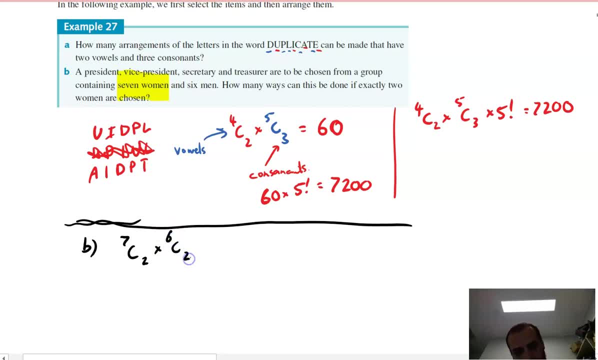 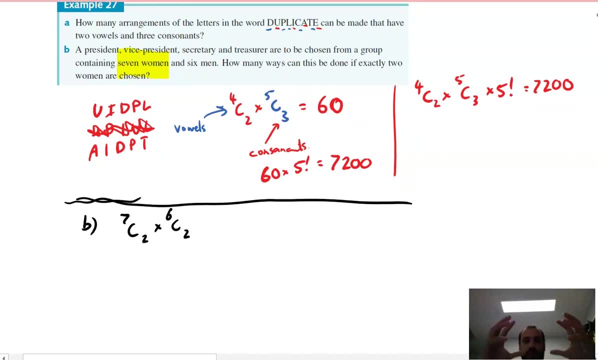 And from the men, from six men, we're going to choose two. Now, that's how many combinations of four people we can get. That's that we know. once we've got those four people, we can combine them as that person. That person's a president. 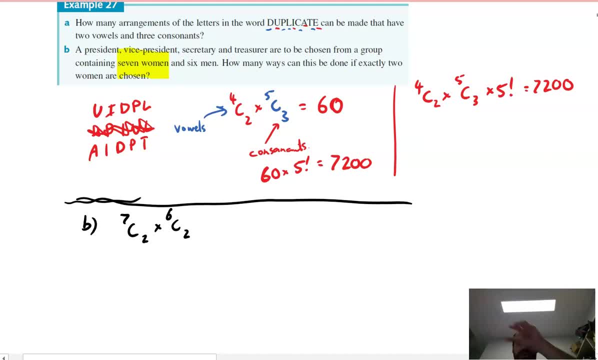 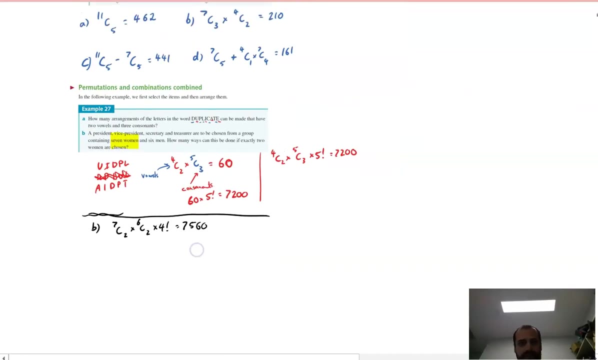 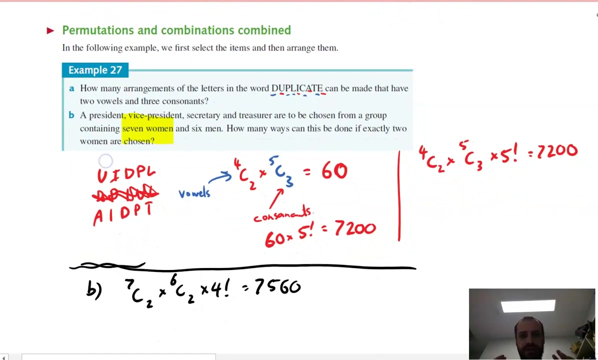 that person's a vice president or that person's going to be the treasurer. We can combine them in four factorial ways. Then there's our answer: 7,560.. Okay, Lots of stuff to consider there, with combinations, with restrictions. but think your way through it step by step, by step. We'll see you next time. Bye. 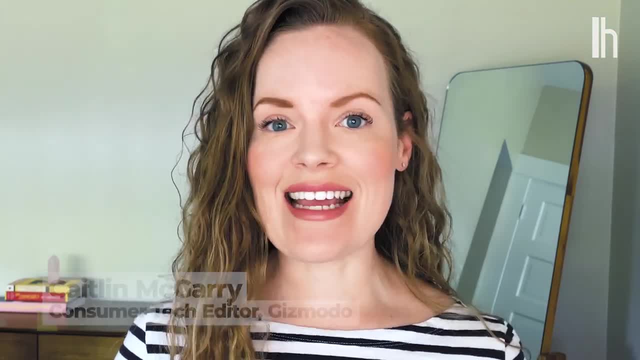 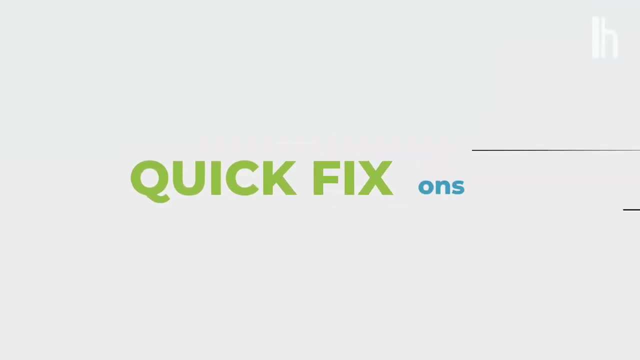 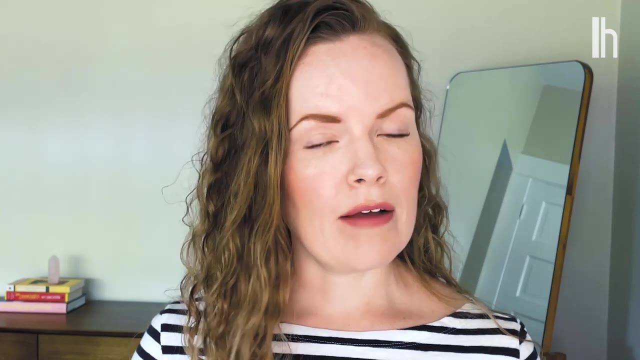 Welcome to Quick Fix, the show where I answer your most commonly asked tech questions in 90 seconds or less. Today we're finally getting around to canceling our subscriptions If you've been paying for apps on a monthly basis or maybe have some auto-renewing subscriptions. 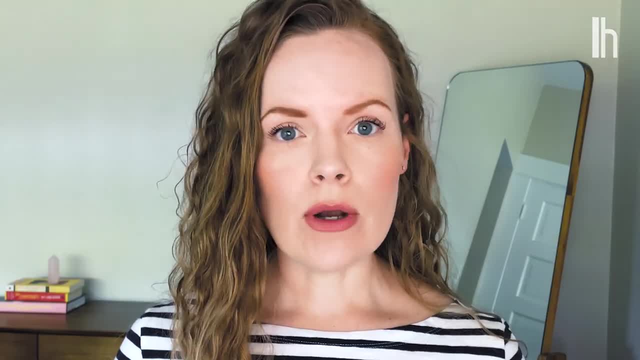 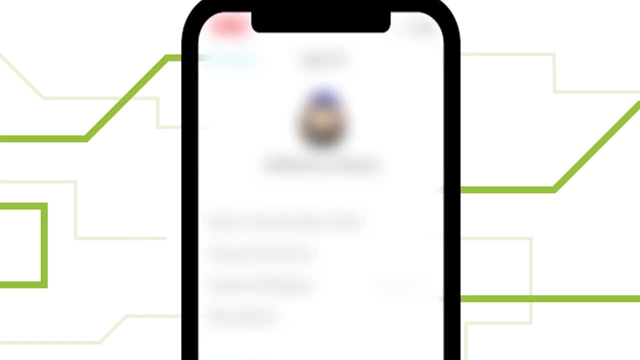 it might be hard to keep track of all your monthly charges. Well, here are four ways that you can easily cancel them. On iOS, go to Settings, Apple ID, then Subscriptions. While you're there, make sure you've turned on Renewal Receipts, so you'll get an email. 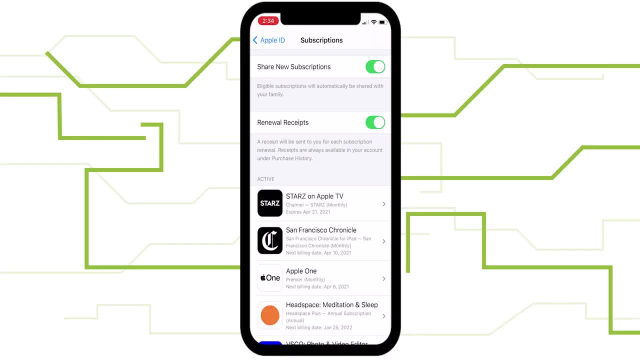 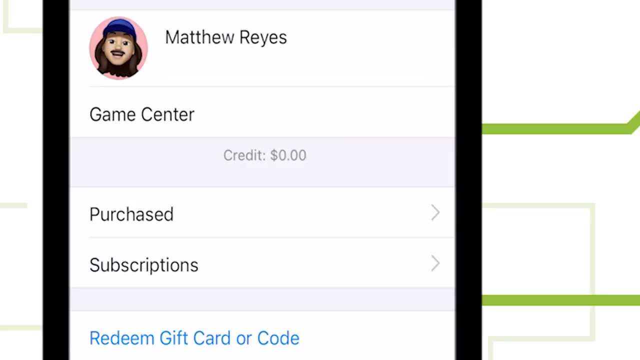 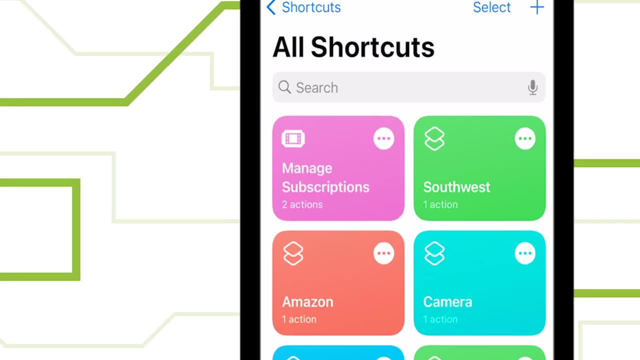 whenever your subscription is about to renew. Now there's no more surprises. You can also go to App Store- Apple ID in the upper right corner and Subscriptions to toggle options. You can even make your own iOS shortcut. Full instructions are below, but you can use this to. access your Apple ID and you'll also be able to purchase a new operating system from Apple. Welcome to Quick Fix, the show where I answer your most commonly asked tech questions in 90 seconds or less. Well, here are four ways that you can easily cancel them On iOS, go to Settings. 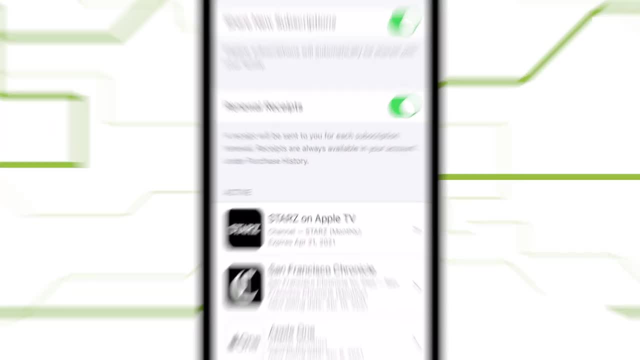 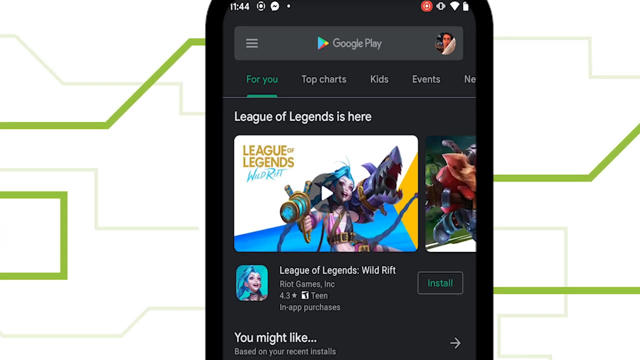 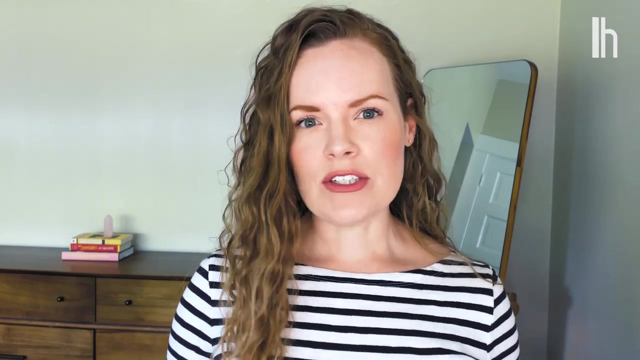 ID and iTunes subscriptions with just one tap. For Android users: visit your Google account's payment and subscription sections. On Android: tap Play Store, the hamburger icon, then Subscriptions. Now your money won't slowly and mysteriously be siphoned away every month. 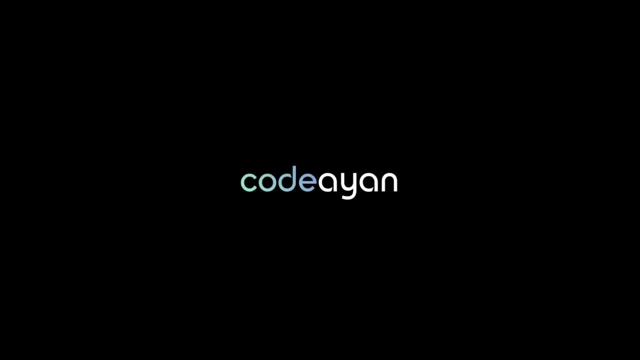 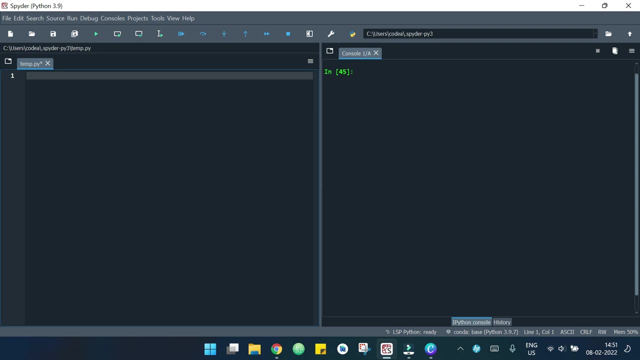 Today we will learn that how to remove an element from a python set. So at first I will declare a set here. Set one is equal to now I will add some elements. Okay, suppose I want to delete this four from here. So to do that I just need to write my set name, which.